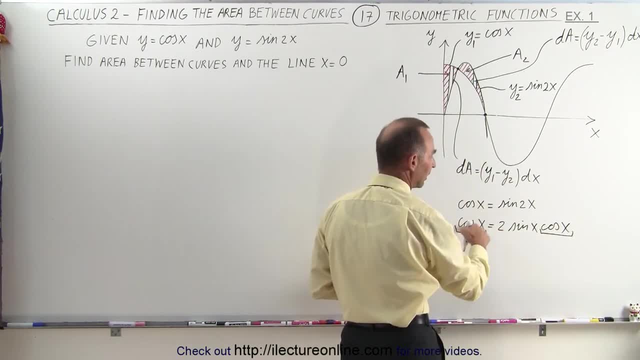 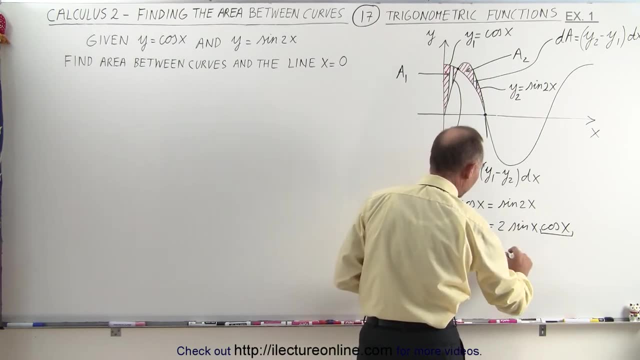 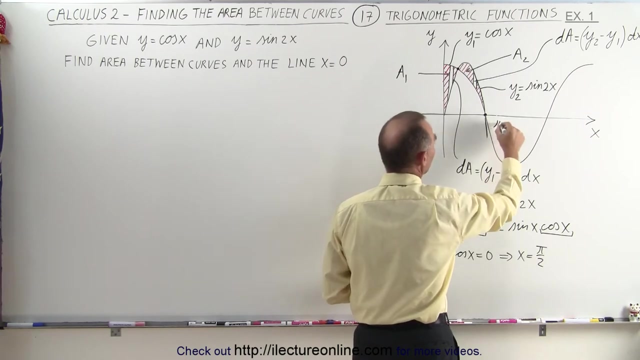 equals the cosine of x. Now, if the cosine of x is equal to zero, then the left side will equal the right side. So one option is that the cosine of x is equal to zero, which implies that x must be equal to 90 degrees or pi over 2.. So that's this point, right here. when x equals pi over 2, then the 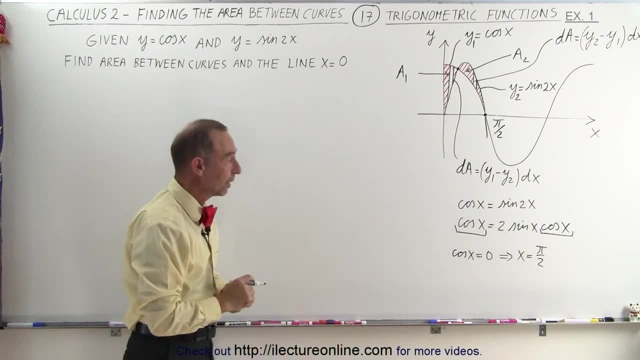 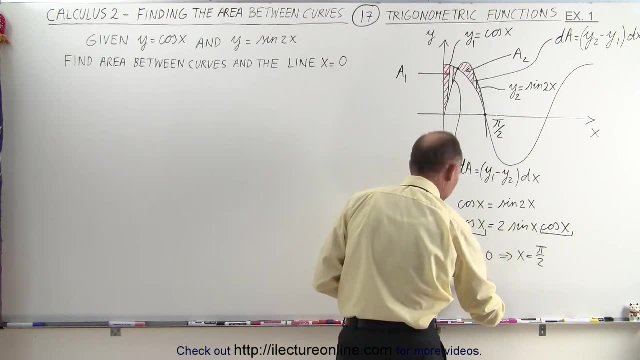 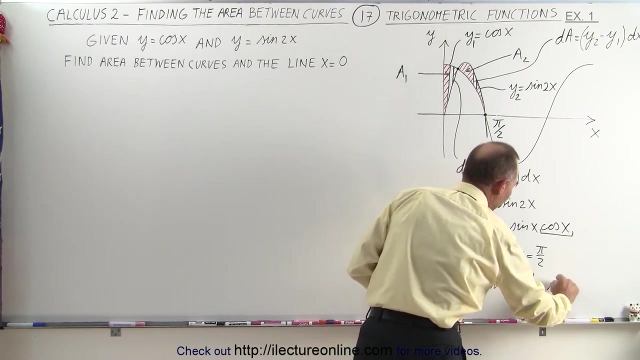 y value is the same for both functions. The second possibility or is to divide both sides by the cosine of x. When we do that, we're going to have to divide both sides by the cosine of x, So we're going to have to do that. We get one equals 2 times the sine of x, or one half equals the sine of x. 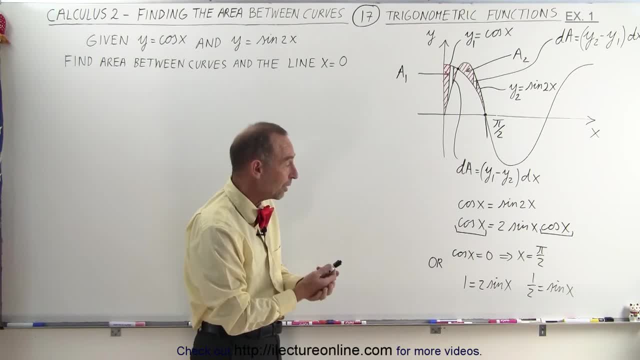 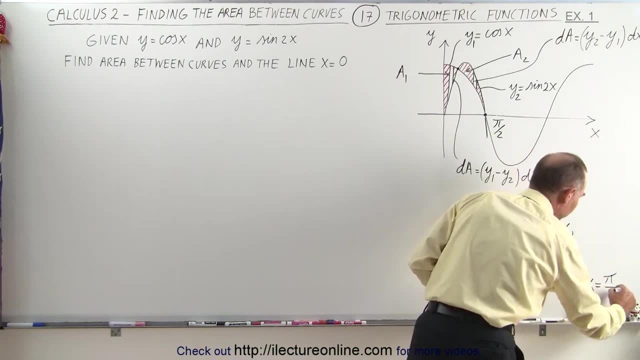 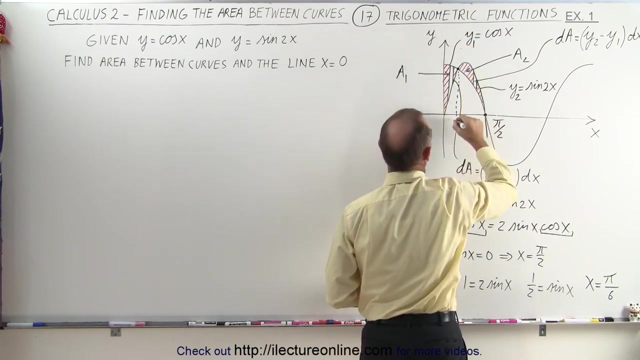 To find the proper value for that. that would mean that the angle x has to be 30 degrees, because the sine of 30 degrees is one half, which also means that x is equal to pi over 6.. So that would be this point, right there. So there we have the point: x equals pi over 6. And x equals the sine of 3.. So 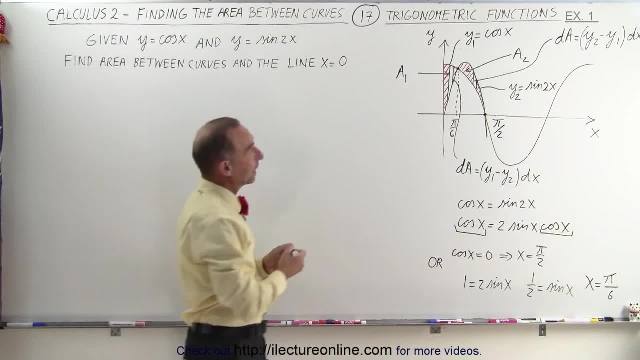 equals pi over 2.. So the limits of integration for A1 is going to go from 0 to pi over 6.. The limits of integration for A2 will be from pi over 6 to pi over 2.. So to find A1: 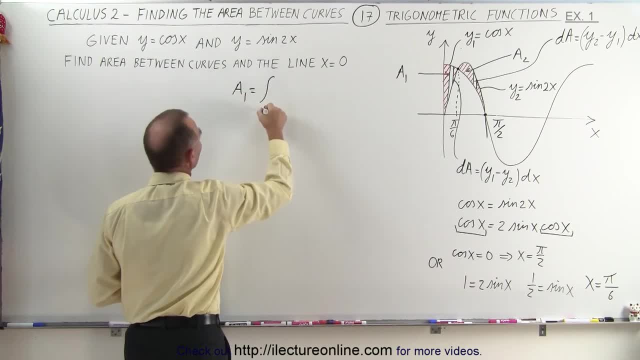 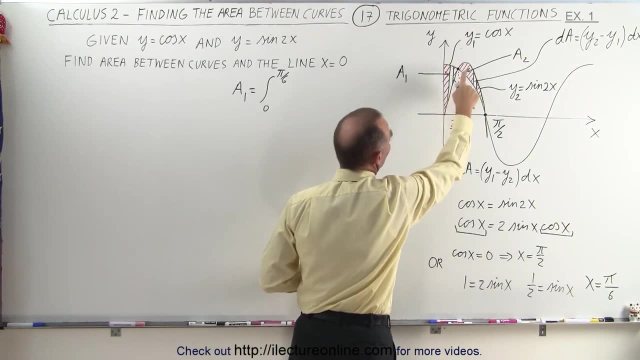 that is equal to the integral from 0 to pi over 6 of y1 minus y2.. So when you want to look at that area element right here, I think I have it defined right here. So dA is going to be y1 minus. 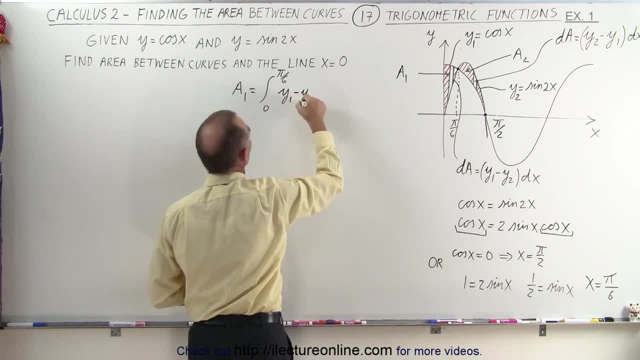 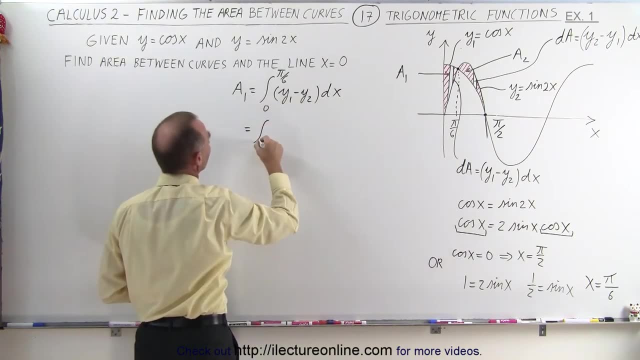 y2 times dx, So y1 minus y2 times dx. and of course these are x limits, and now we will plug in what these are. This is equal to the integral from 0 to pi over 6 of y1, which is a cosine of x. 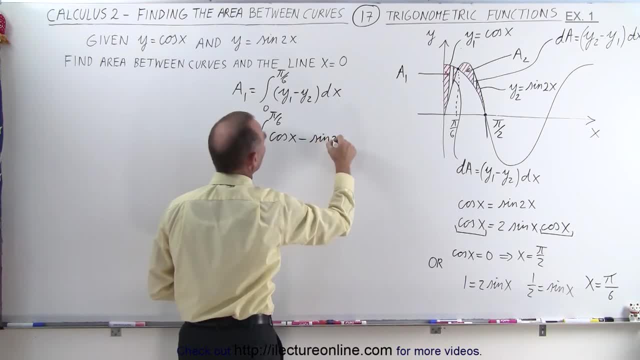 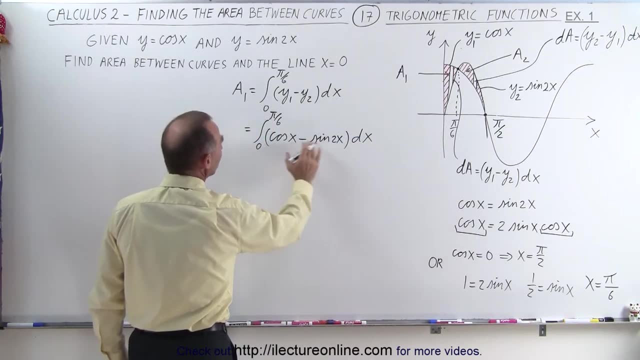 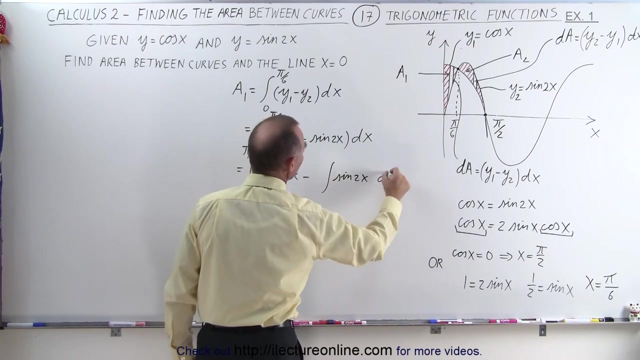 minus y2, which is a sine of 2x times dx. So when we integrate this we really should break this up into two separate integrals. So this becomes equal to the integral from y1 minus y2 times dx, from 0 to pi over 6, of the cosine of x- dx and then minus the integral of the sine of 2x dx. 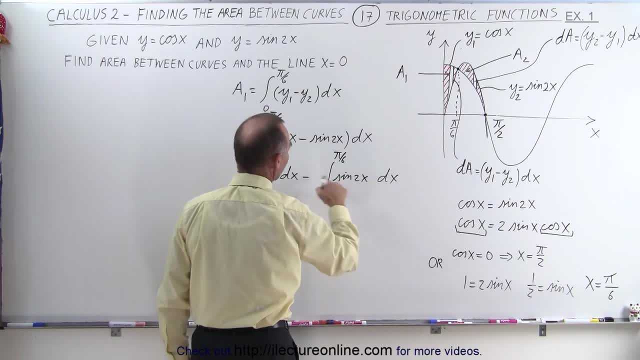 from 0 to pi over 6.. Notice, I left a little bit of room here because we do have to find the proper differential To integrate the sine of 2x. we're going to need a 2 dx, so that means we need a 1. 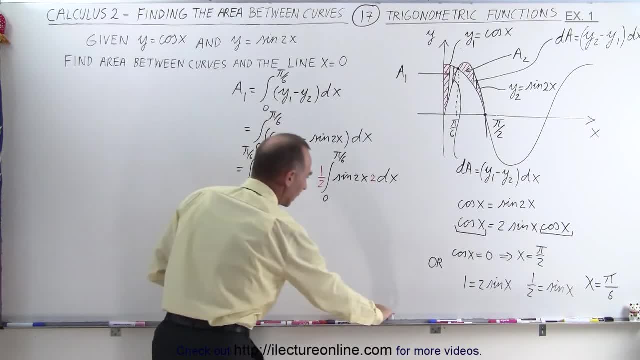 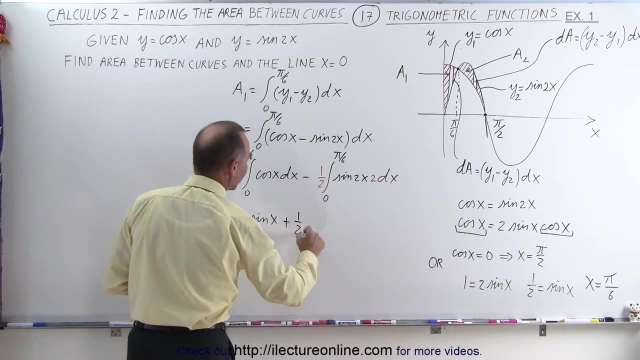 half in front to compensate for the 2 that we put in there. and then the integral of the cosine is the sine. but the integral of the sine is the negative cosine, so this will negate this negative sine, become positive. so this becomes equal to the sine of x plus 1 half times the cosine of 2x. 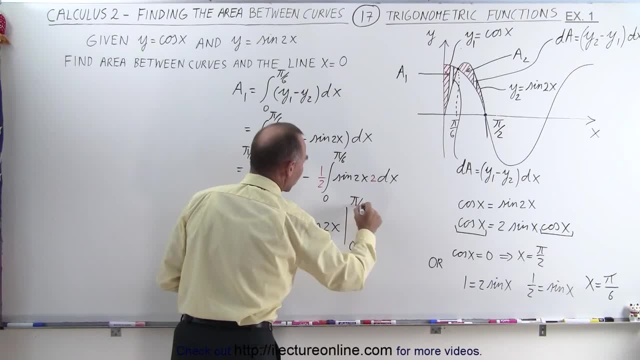 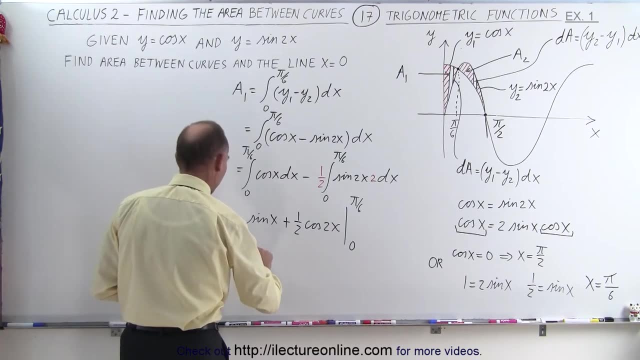 all evaluated from 0 to pi over 6, since the limits of integration are the same for both. So we'll plug in the upper limit. we get the sine of pi over 6 plus 1 half times the cosine of 2x. So we have a cosine of 2 times pi over 6, which is pi over 3, and then subtract from that when we plug. 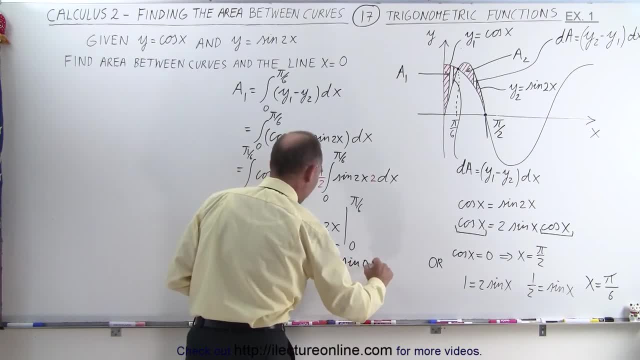 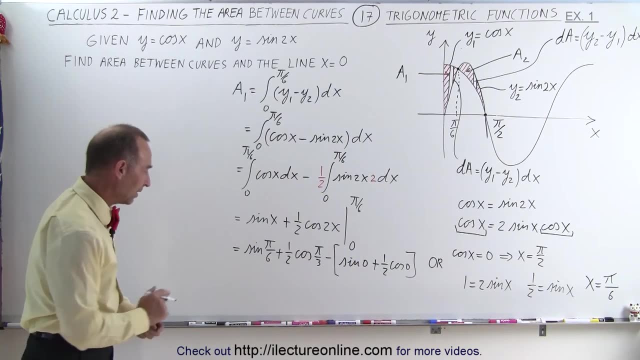 in the lower limit, the sine of 0, which of course is 0 plus 1 half times the cosine of 0, and I think now we can evaluate this: the sine of pi over 6. that would be equal to 1 half, because that's the 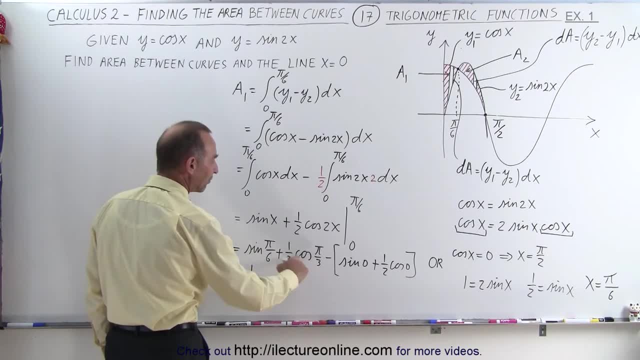 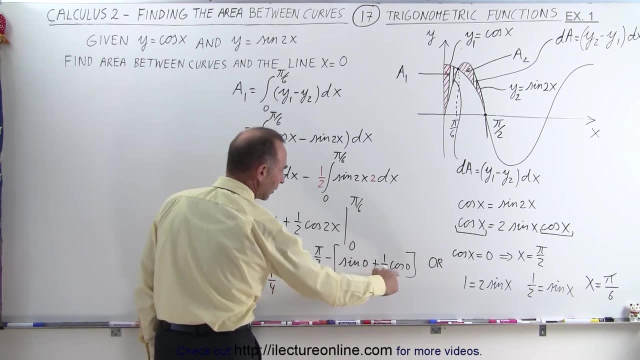 sine of 30 degrees, the cosine of 60 degrees is 1 half times 1 half is a fourth, and then we subtract from that minus 1 half times 1, half times 1 half is a fourth, and then we subtract from that minus, the sine of 0 is 0. but here the cosine of 0 is 1, 1 half times 1 is 1 half, and subtract 1 half from. 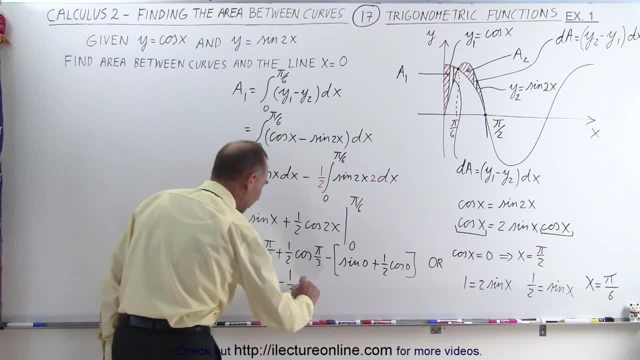 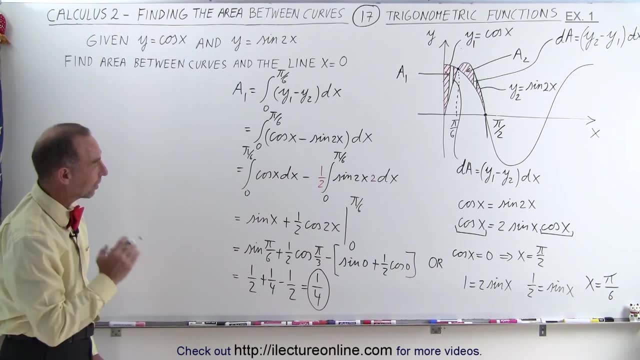 that. so that's 1 half, and notice 1 half minus 1 half cancels out and we get 1 quarter for area 1. so for the first area, from 0 to pi over 6, that is equal to 1 quarter. Now we need to find the area. 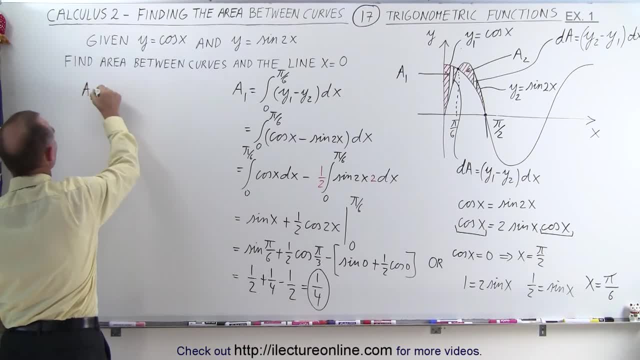 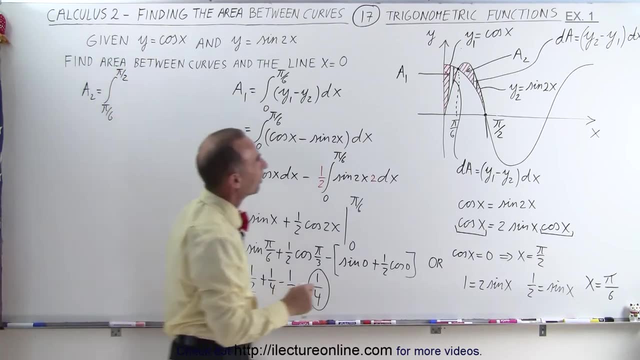 a2. so let's do that over here. so a2 is equal to the integral from pi over 6 to pi over 2.. And notice, in this case the area element da here is defined as y2 minus y1, it's in reverse, so that 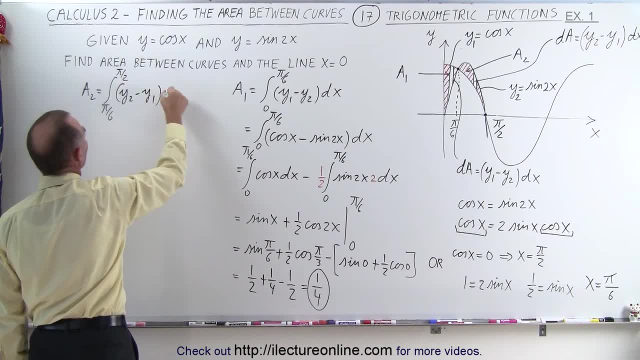 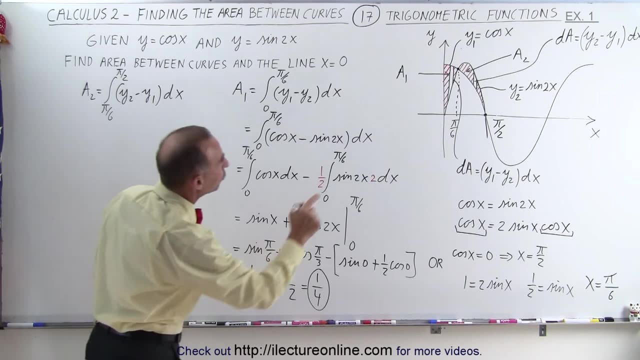 would be y2 minus y1 times dx. of course these are x limits, and then we plug in what y2 and y1 are equal to. so y2 is equal to the sine of 2x. so this becomes equal to the integral of the sine of. 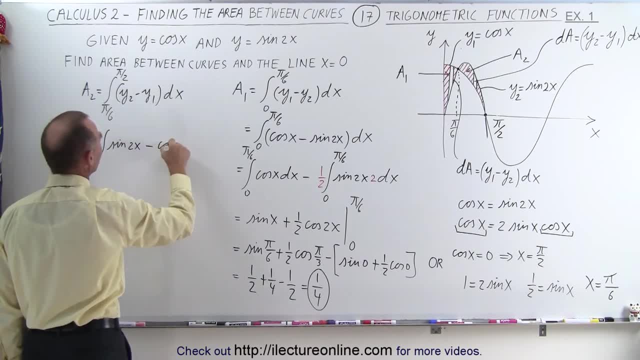 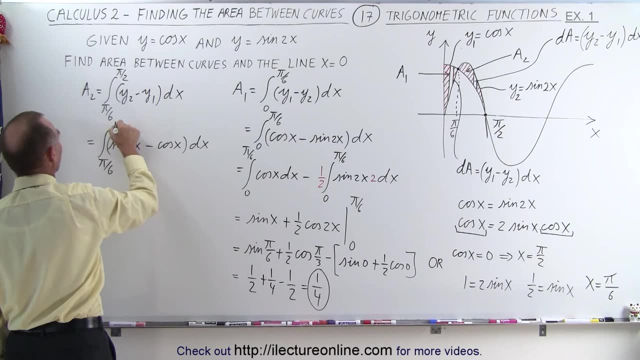 2x minus y1, which is the cosine of x times dx, And from pi over 6, this is a 6 right here to pi over 2.. So now we're going to write this again like two separate integrals. 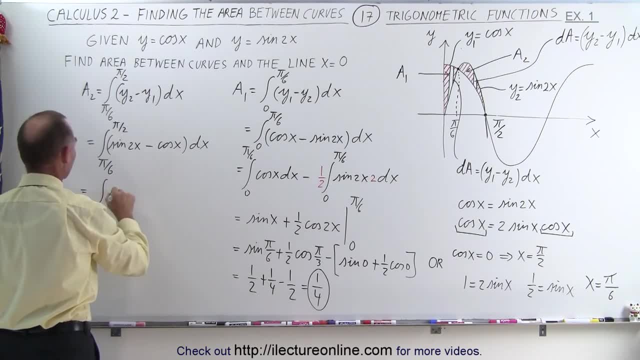 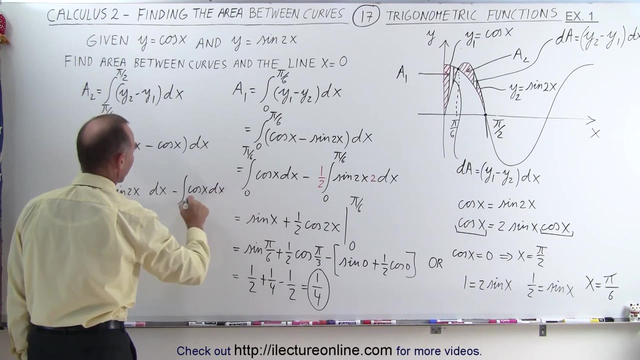 So this becomes equal to the integral of the sine of 2x times dx- And notice I left a little space in here- from pi over 6 to pi over 2.. And then minus the integral of the cosine of x times dx, again from pi over 6 to pi over 2.. 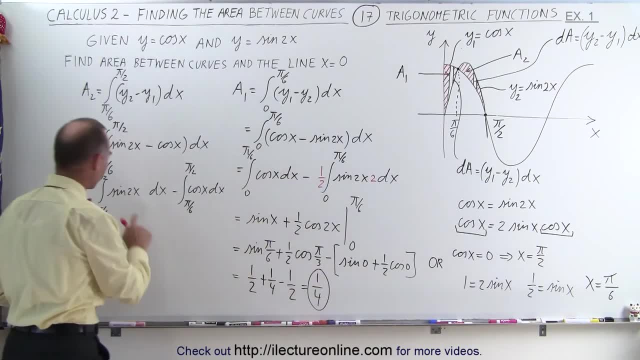 And now, the reason why we left a little space is because here I need the proper differential to the x and I need a one-half here to compensate. So now I'm ready to integrate both integrals, This one here, the sine of 2x, so we integrate. we should get the negative cosine of 2x times one-half. 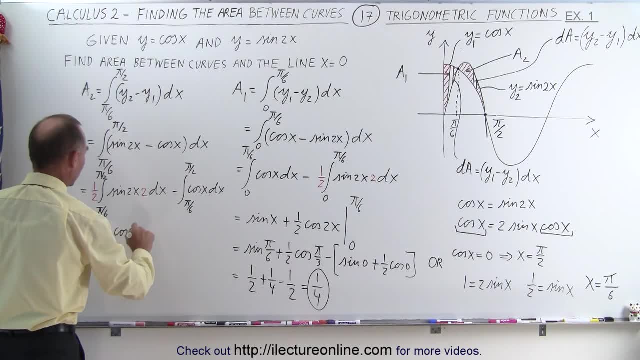 So this is equal to minus one-half times the cosine of 2x, And then here the integral of the cosine is the sine, but we have the negative in front here. so that's minus The sine of x, evaluated from pi over 6 to pi over 2.. 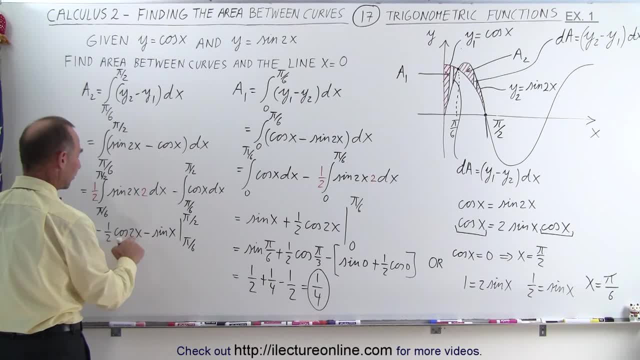 So now let's plug in the upper limit. We're going to plug in the cosine of 2 times pi over 2, so we have minus one-half times the cosine of 2 times pi over 2, which is pi Minus the sine of pi over 2.. 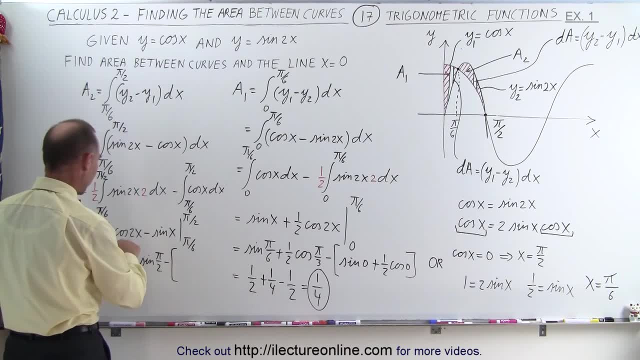 And now subtract from that when we plug in the lower limit, So we have one-half here We have a minus one-half times the cosine of twice pi over 6, which is the cosine of pi over 3.. 3 I should have. 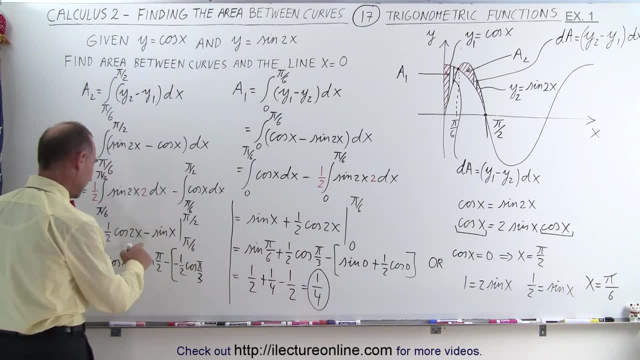 Let me put a line over here so we don't get confused here. And then we have a minus. We plug in the lower limit here, so that would be upper limit minus the lower limit. So we have the sine of pi over 6 to the sine of 30 degrees.